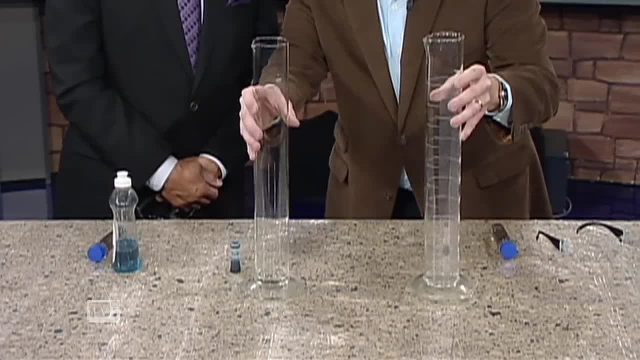 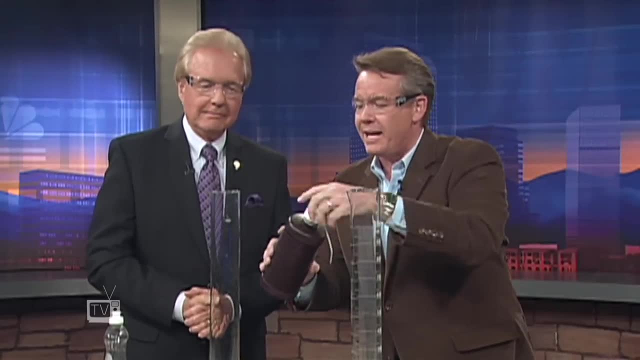 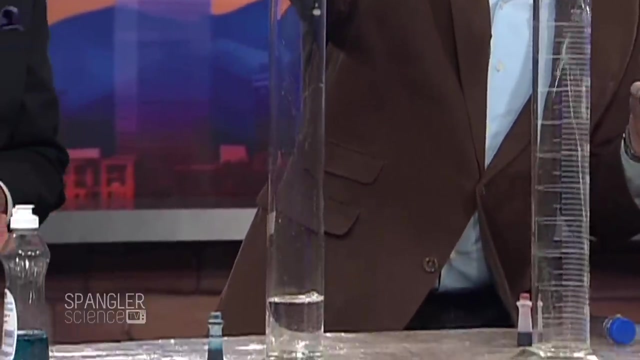 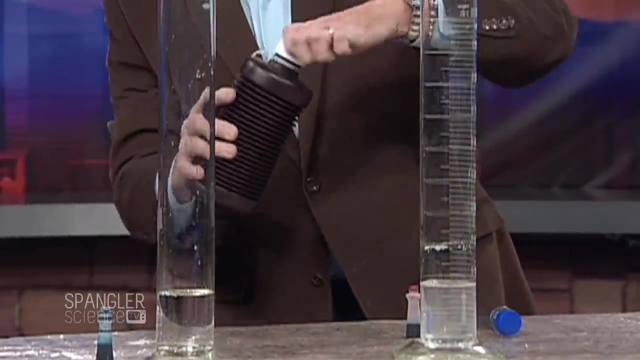 And it's tall and has structure, It's support, It's clearly transparent. You know how that works. Yeah, Put on your safety glasses, because we always practice safe science, We do- And a little bit of liquid goes down inside, of course, representing the students that you don't tell them early on that this is hydrogen peroxide. Oh well, of course. Of course it is. So it all runs in terror. It's exactly right. So this is our hydrogen peroxide. Now, the nice thing about hydrogen peroxide is it's H2O2, which means it's water and oxygen. So it represents all the students that could ever ever be there, Right? 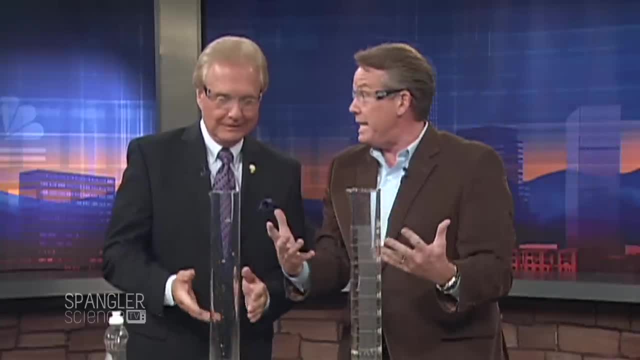 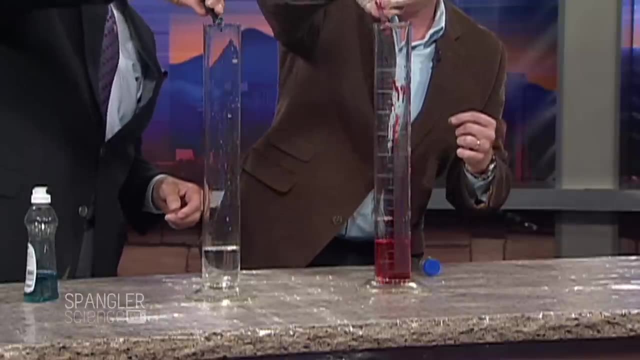 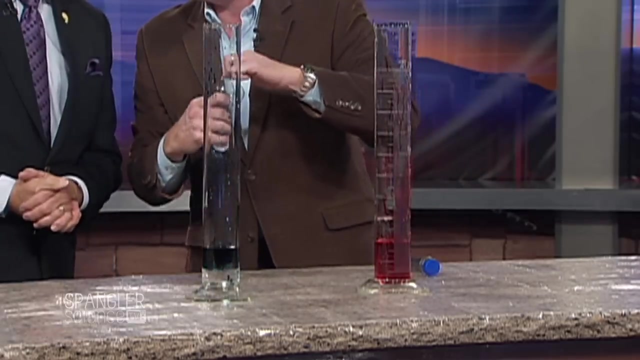 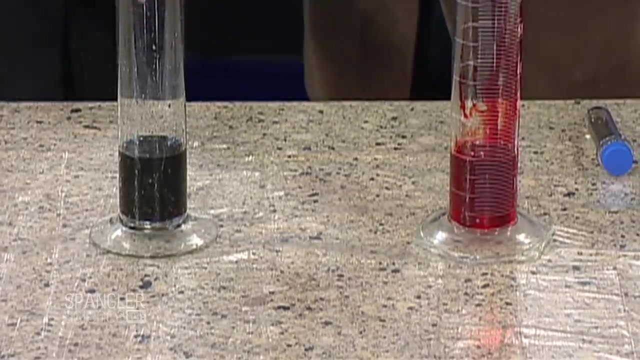 They look like kids early on. There's tremendous enthusiasm. You just have to get it out of them. Correct, Right? All kids are different. So here, take your food coloring. No, no, Take your food coloring. Oh, food coloring. Push the food coloring inside like this. That was almost a disaster, wasn't it? No, no, It's perfect. That was perfect. So all kids are different. So we have to put that in there. And if you're going to do something in school, they have to have a way to measure success, And so a little bit of soap is going to help us measure the success, like this. So now, Look how much neater mine is than yours. I know I'm a little sloppy that way. Yeah, you are. Yeah, So the coolest thing that could ever happen with a teacher: take your test tube and take the lid off, Okay. 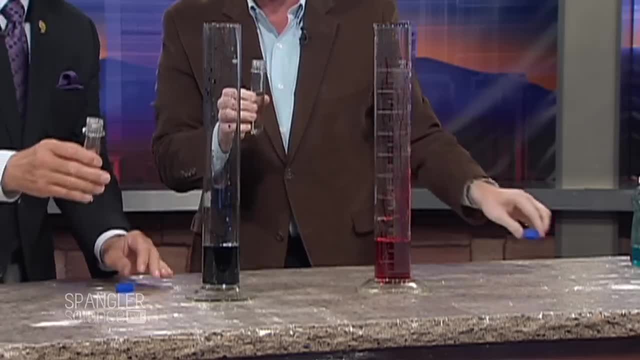 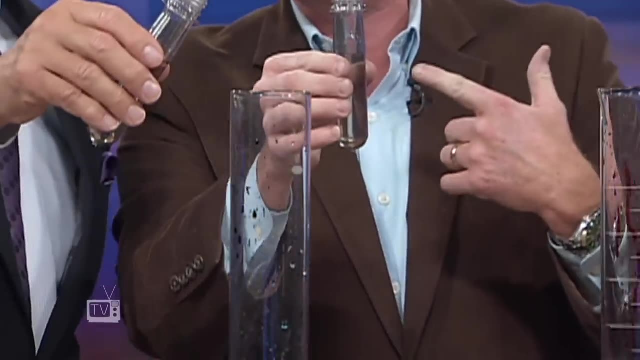 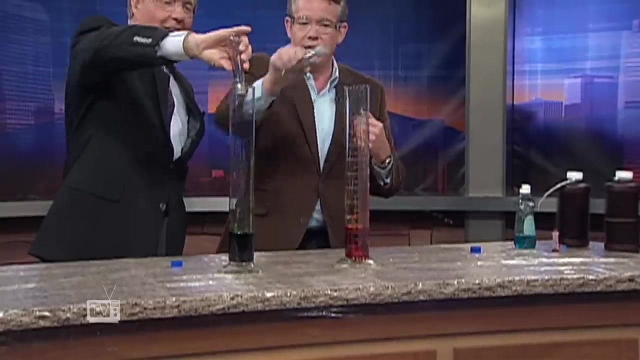 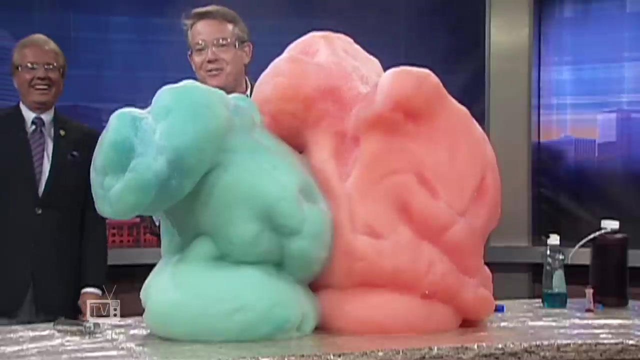 Is this? A teacher acts as a catalyst, And that catalyst tries to get kids to come out of their shell. And if you want to see what a great school is like, Do I need to run after I? I don't know that running is a thing, But here's what I would do. I think I would do a wide shot. You know what I mean? Oh, I think I would go wide. Oh, okay, So you can see what's going to happen. Ready, Here we go, Mark, Okay, Releasing enthusiasm. Three, two, one. go Dump it in. Nice job. This is just, Oh, hello, This is, This is the overflowing enthusiasm of any kid on the first day of school. Look at this. We didn't know it was inside, But in the hands of a great teacher, it erupts And everyone's like, Oh my gosh. 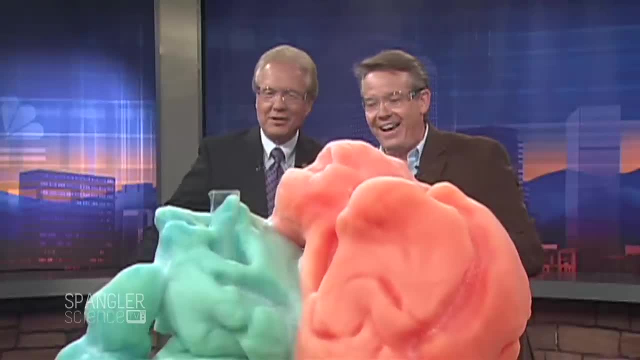 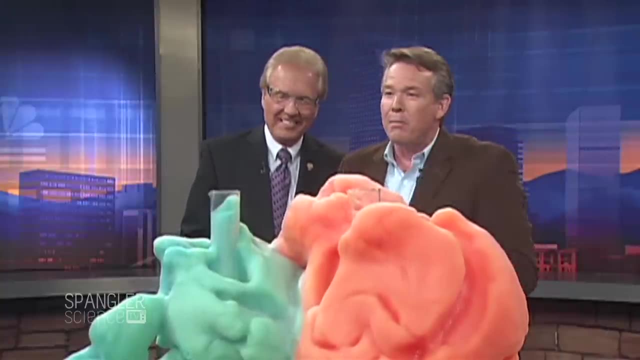 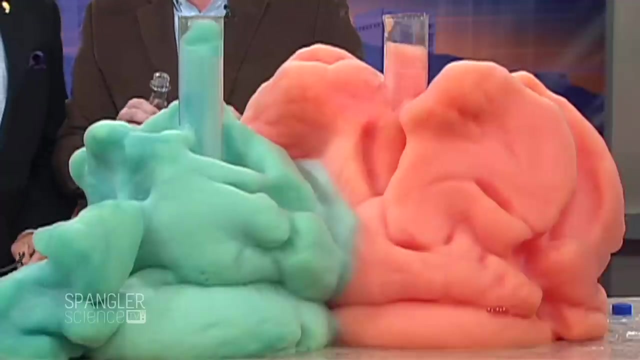 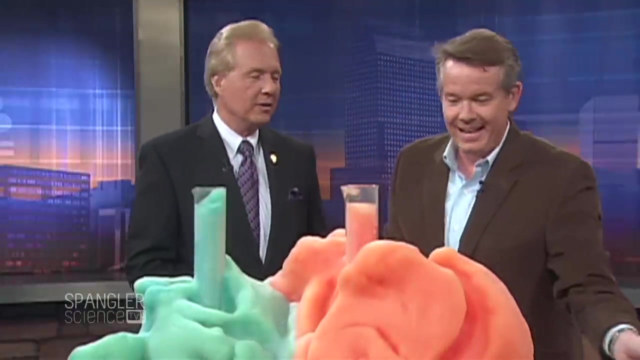 Every parent goes. I'm so happy There goes another suit. We release energy. It's what happens on the first day of school. So, as I look into the camera right here and say, moms and dads, please ask kids what happened on the first day of school. It's the most important question you could have And you never let them say nothing. They always learn five things that they never knew before. And this is what happens in the hands of a great teacher. That's great fun. I also like to point out that the twins are in middle school now, which is also It's a big night at the Spangler.